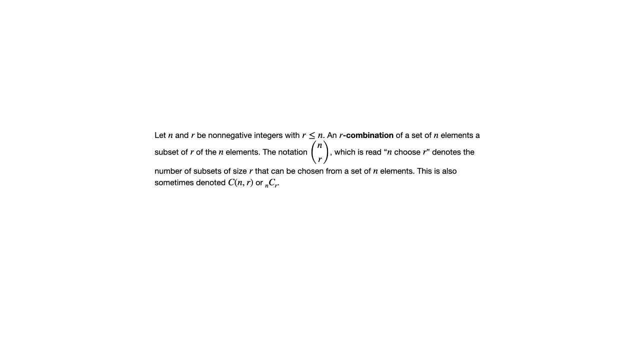 size r that can be chosen from a set of n elements. There's some alternative notation given here. The formula which we first saw in chapter 5, is n- factorial over n minus r factorial. Okay, so a couple of notes I want to make about this before we move on to the other concept, that's 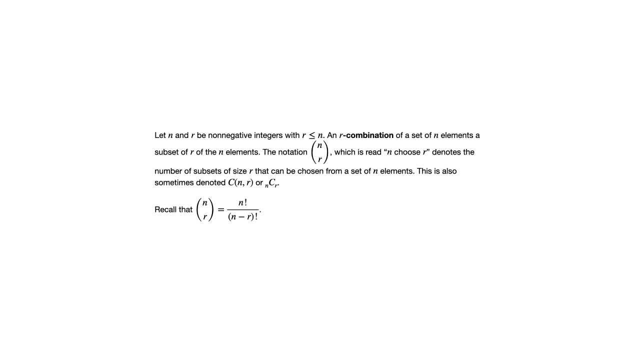 highlighted in this section. First of all, here we can use this new rule now to fix scripts along with the other rules that we've seen in chapter 9.. So you're going to see this in the exercises used along with the multiplication rule or along with the addition rule, And so now that we have 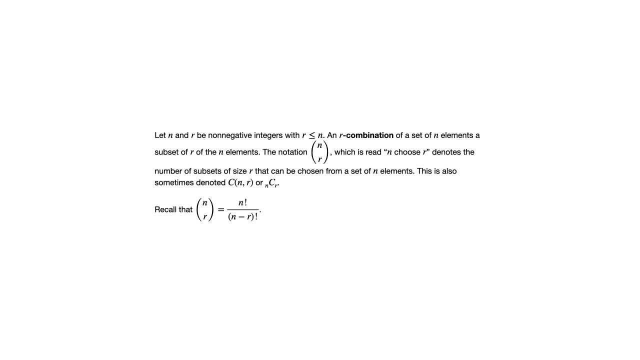 all kinds of tools that we learned in chapter 9, we can look at some pretty interesting examples, And I think you'll want to look at the exercises for section 9.5 next. you'll see that they're, they can be quite interesting examples, and you know. 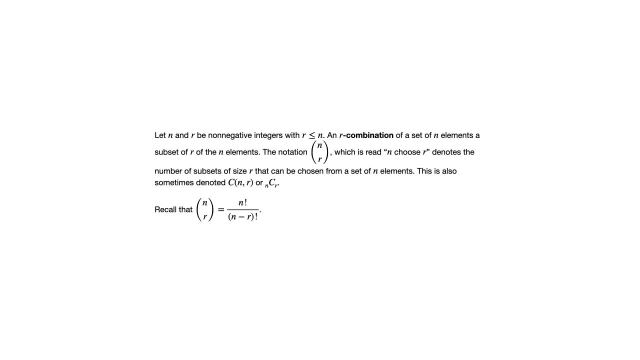 seeing the various ways that these rules work together. A couple other things I want to note here. One is that, remember, with combinations the order does not matter, We're just talking about subsets of a certain size, Whereas with permutations the order does matter, And that's what distinguishes those two. 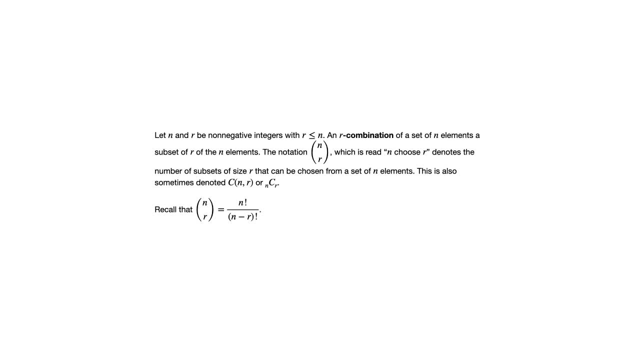 concepts. Their formulas look pretty similar. So if you're ever in doubt, just think about whether the order matters or not. The other thing I want to note here is, as I mentioned in a previous video when we were looking at permutations, any scientific calculator is going to have some kind of function key. 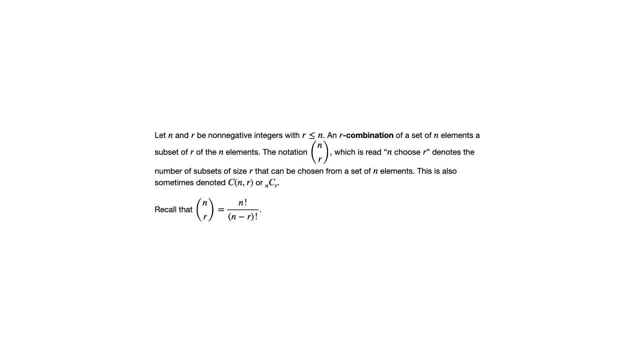 that will handle combinations, And nearby you'll have something that does permutations, And nearby you'll have something that does factorials. Those three things tend to be grouped together. They might be in a menu somewhere or a shift of another button, But that can be useful to have in mind, especially when 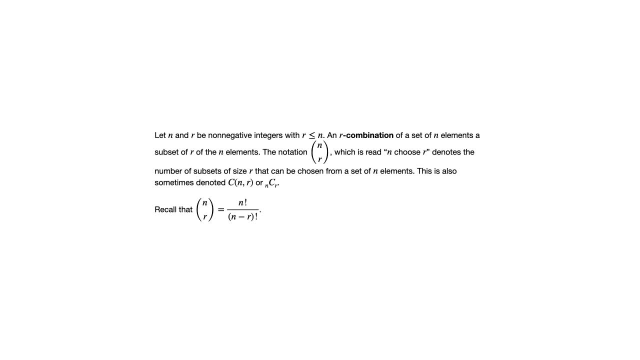 some of the numbers are more difficult to work with if you didn't have the right calculator. So keep that in mind and I encourage you, if you're not already sure where that's located on your calculator, to take a moment to kind of look into that. Okay, something new that's presented to us in this section is 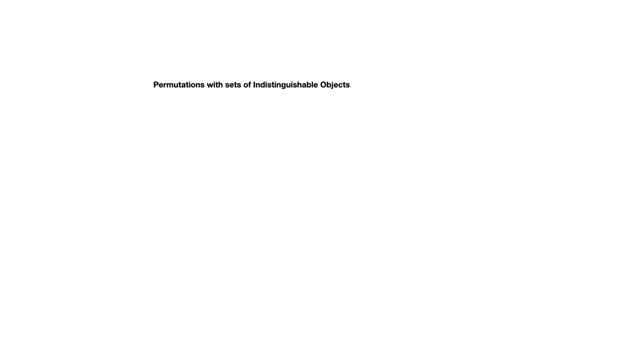 permutations with sets of indistinguishable objects, And let me explain what that's referring to, and then we'll get to the final part. Okay, permutations is a formula. So if you took a word, let's say that has some letters that are repeated, and you were to scramble those letters. Well, that, 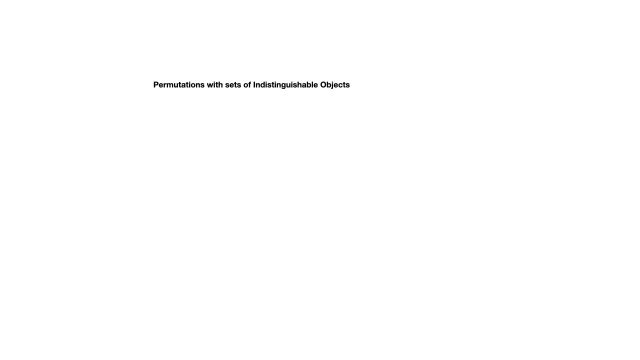 would be a little bit different than scrambling the letters of a word where all the letters are different. Okay, so if you have some letters that are repeated, that's going to be different than if all the letters are distinct from each other. And so, for example, if the 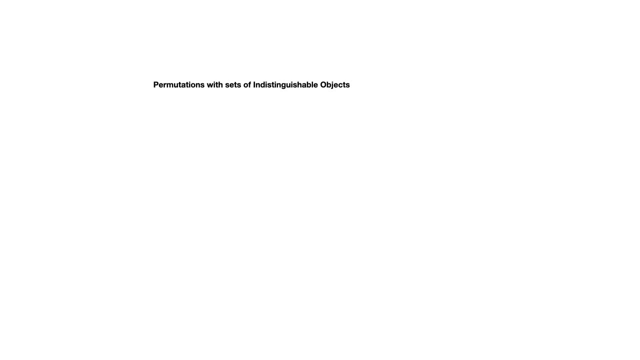 word has two T's in it and you just swap those two T's around. well, you haven't really changed anything in terms of how that word looks right. So what we want to do is be able to come up with a way of counting the different arrangements of. 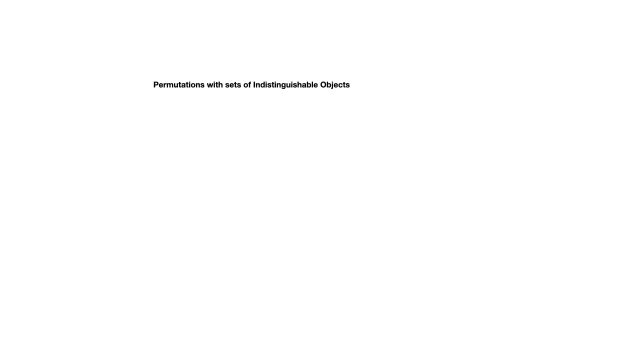 those letters, but keeping in mind that some of the letters are the same, so scrambling those among each other does not change anything and should not be counted as a separate order, a separate permutation. So here's the formula. So if you have n objects to start with, and let's say n, 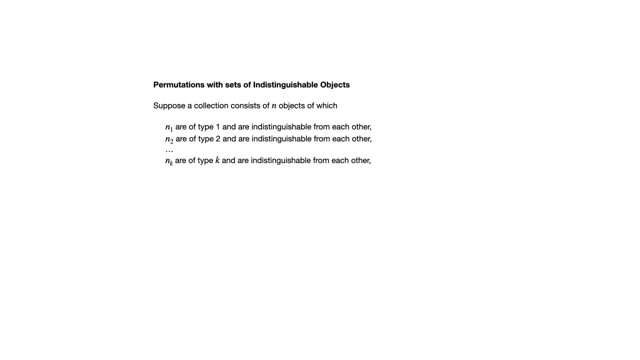 sub 1 are of the first type and n sub 2 are of the second type and n sub k are of the kth type, and n is the sum of all those n sub 1 through n sub k, then the number of distinguishable.